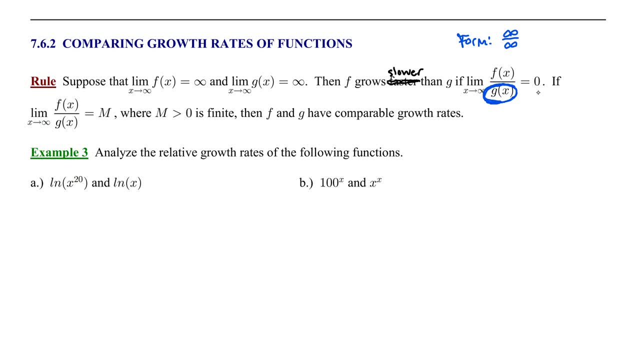 memorize this rule. Now here's where it gets interesting. If the limit, as x approaches infinity, of the ratio of f divided by g is m, where m is a positive number and it's finite, then f and g have comparable growth rates. 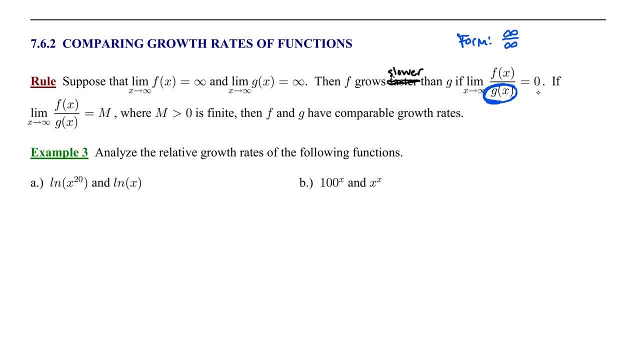 And that limit m is going to tell us how those growth rates relate to each other. In example three we want to analyze the relative growth rates of the two given functions. Example a: natural log of x to the 20th and natural log of x. 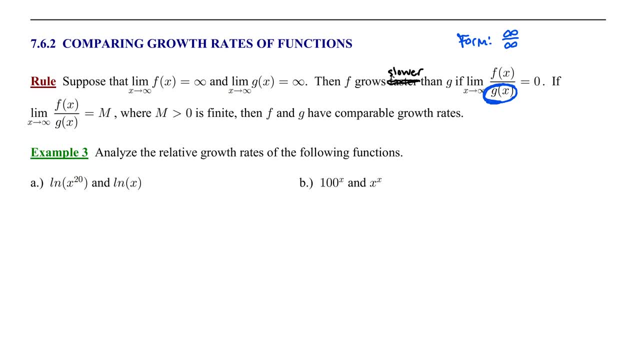 Notice, both of those functions have a limit at infinity. that equals infinity, That is, both of those functions grow without bounds on the far right side of their graph, But we want to know who grows faster. I don't know about y'all, but my bet is on this first one. 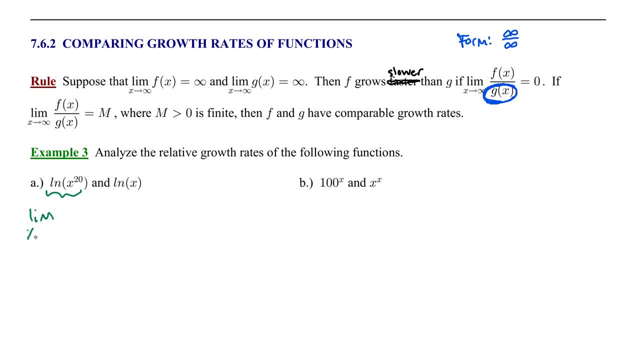 But let's prove it, Let's be specific. So let's find the limit, as x approaches infinity, of the ratio of these two functions. Now, if you learn how to interpret this, you'll be able to find the limit, as x approaches infinity, of the ratio of these two functions. 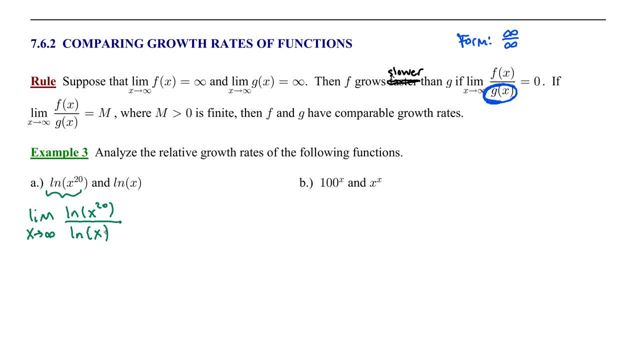 Now, if you learn how to interpret this limit, you can put those in any order: Natural log of x to the 20th, on top or on the bottom. Now we have the form infinity over infinity And of course that gives us the green light for L'Hopital's rule. 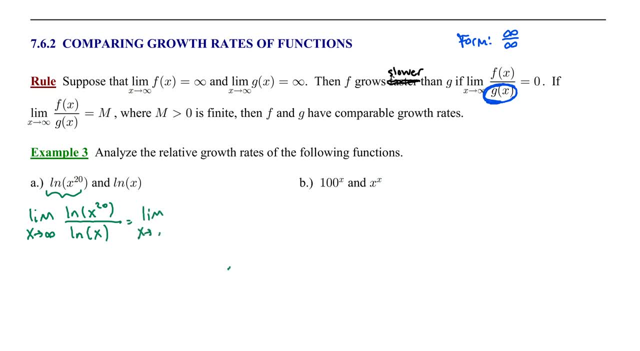 So we'll individually differentiate the numerator and the denominator. So in the numerator I'm going to put the argument, in the denominator and the derivative of that argument in the numerator. And in the denominator we're going to find the derivative of natural log of x to the 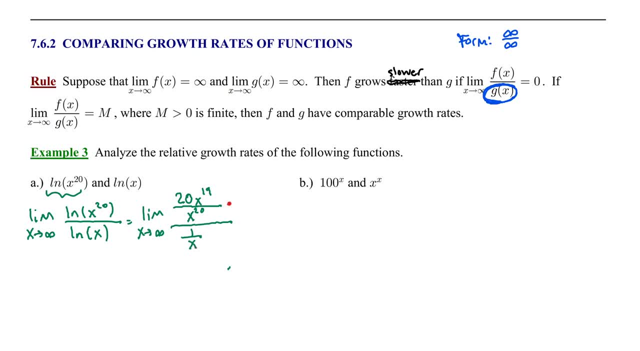 20th over x, which is 1 over x. Now let's do some algebra to cure this complex fraction. here We're going to multiply both the top and the bottom by x, So that's going to clear the denominator, And we can simplify this to the limit as x approaches infinity of 20.. 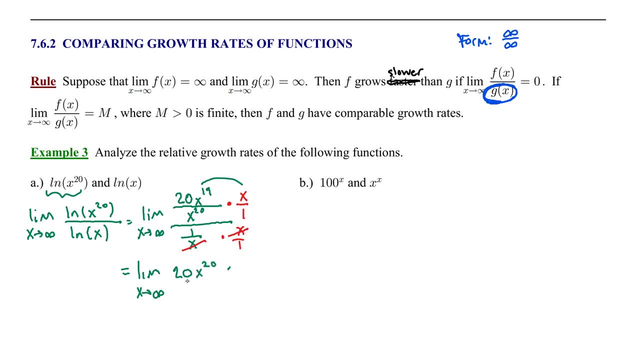 And notice, if we multiply these numerators we'd have x to the 20th over x to the 20th, where of course those x to the 20th cancel. So now we're looking. We're looking at the limit of a constant. 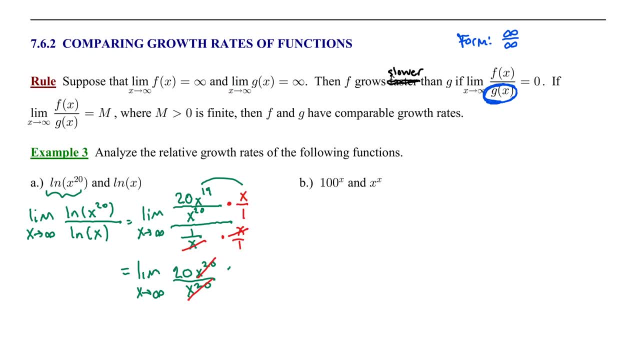 The limit of a constant is a constant. Thus the value of this limit is 20.. Now, since natural log of x to the 20th was on top, we can say that natural log of x to the 20th grows 20 times faster than natural log of x. 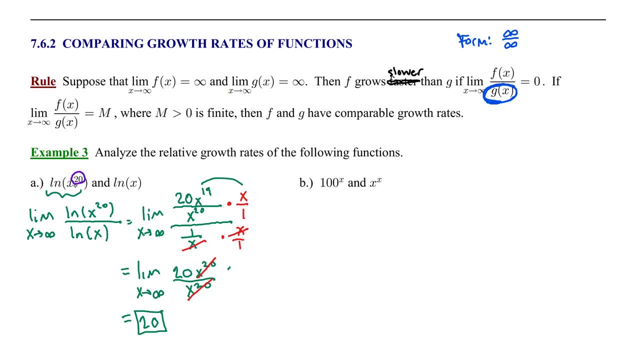 And doesn't that make perfect sense? If I take this exponent and apply log properties and move that down as a coefficient, I can clearly see that the value of x to the 20th is 20.. I can clearly see that the first function is 20 times the second function. 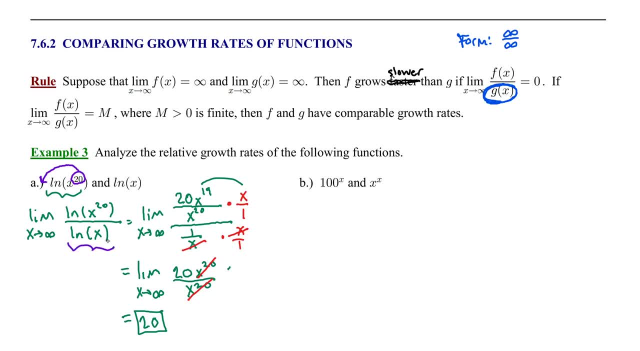 Now you may have seen that all along, You may have thought to apply that right here, And if you had moved this exponent and calculated the limit without doing all of these calisthenics, you would have still ended up with a limit of 20.. 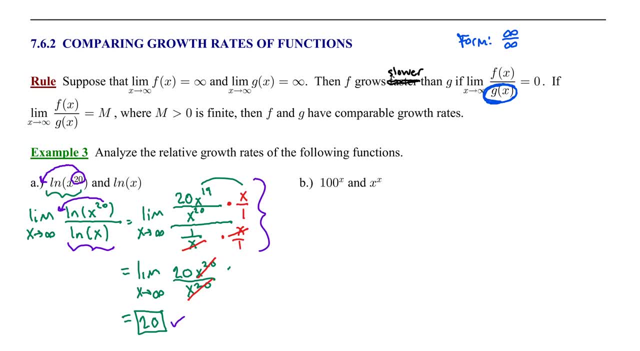 So if you thought that, great job, Now here's a good question: Who grows faster, 100 raised to the x power or x to the x power? Well, let's find out. Let's find out by taking the limit at infinity. 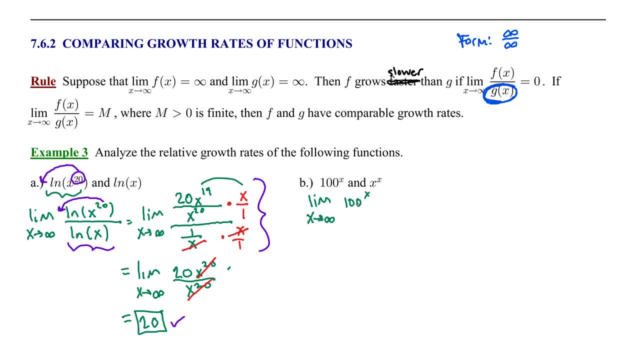 So the limit, as x approaches infinity, of 100 to the x divided by x to the x- Well notice, our indeterminate form here- is still infinity over infinity. Now, if I want to apply L'Hopital's rule directly, that means I'm going to need to: 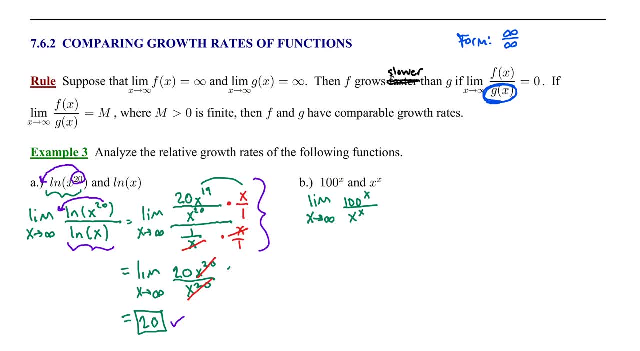 differentiate x to the x power. We have done that in a previous video, in our notes, but you may not have memorized it. So if you don't have it memorized, what are you going to do? Well, here's another option. 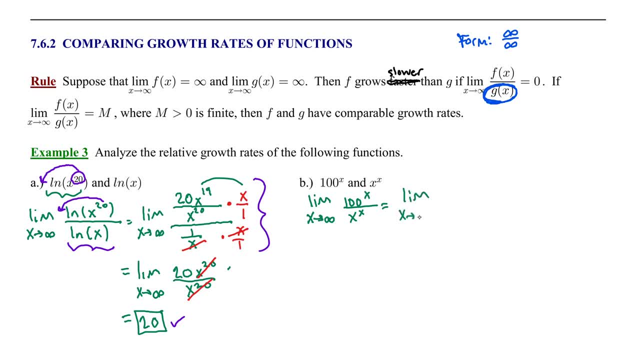 Let's rewrite this as the limit as x approaches infinity of 100 divided by x raised to the x power, because they both share that common exponent. Then let's go ahead and introduce the left side. Let L equal the limit as x approaches infinity of 100 divided by x raised to the x power. 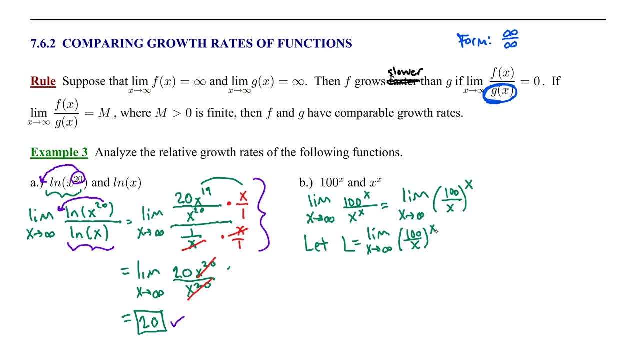 We're going to make use of logarithms to calculate this limit. Observe, If that we have a variable base and a variable exponent. generally, in that situation we need to use logarithms to execute the limit. So let's go ahead and take the natural log of both sides and, as we have seen previously, 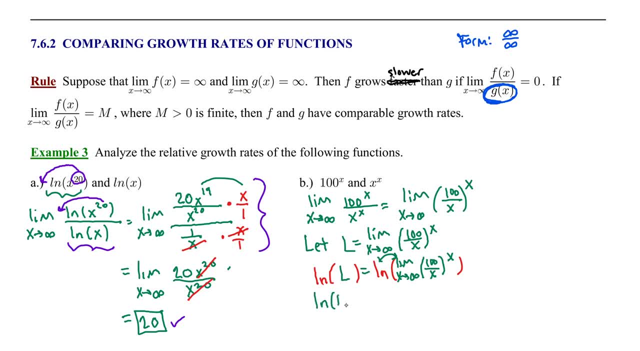 we can reverse the outside function and the limit operator So that we have the limit as x approaches infinity, of natural log of 100 divided by x raised to the x power. Then, as we've been practicing, we can take the exponent on the argument of that natural log. 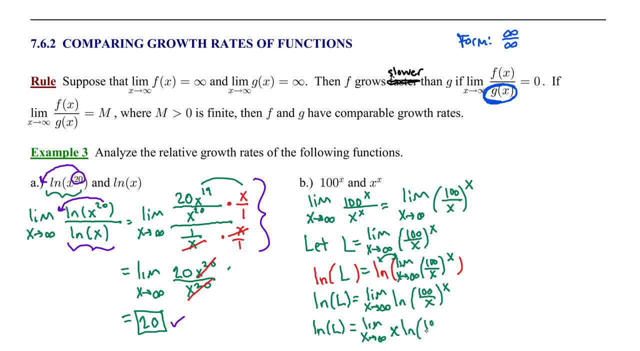 and move it down in front as a coefficient. Now, thinking about x approaching infinity, this first little factor: x approaches infinity as x approaches infinity. and here we have x approaches infinity as x approaches infinity. And here we have x approaches infinity as x approaches infinity. as x approaches infinity. 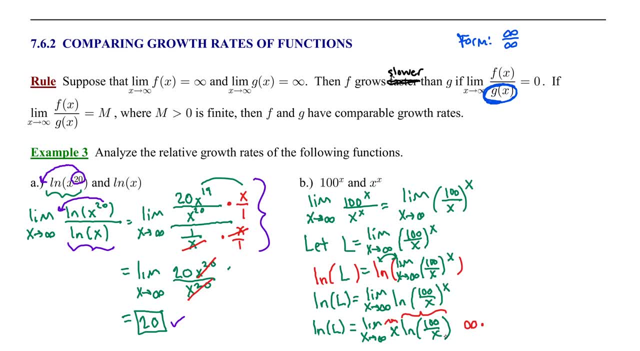 have natural log of 100 divided by x. Well, as x approaches infinity, the argument approaches 0, and as the argument approaches 0,, we know that natural log approaches negative infinity. Now, infinities can be tricky, but not in this case. If you have a factor approaching infinity. 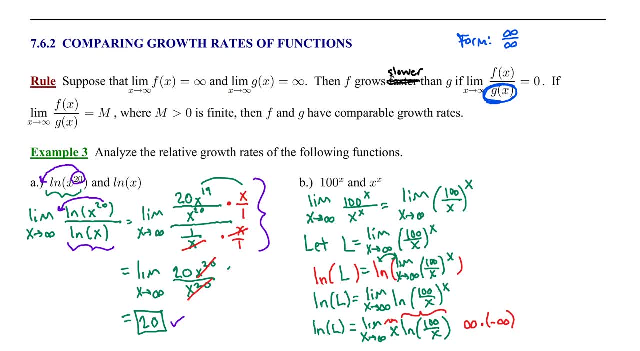 times another factor approaching infinity. I'm going to ignore the negative for a minute. Well, infinity times infinity, that's just going to give me a really big number, right? So infinity times infinity is infinity. Infinity behaves weird sometimes, By the way. 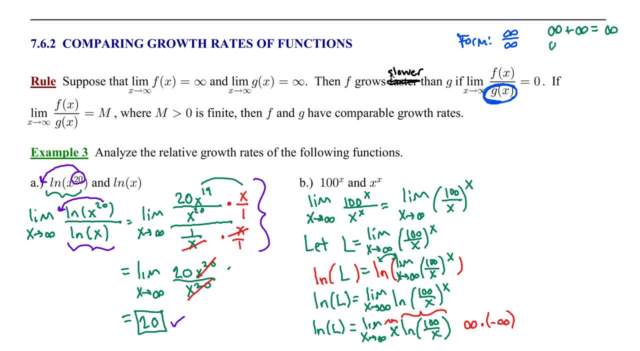 infinity plus infinity is infinity, but infinity minus infinity is not necessarily 0. if they're growing at different rates Infinity times, infinity is infinity, but infinity divided by infinity is not necessarily 1.. We know that's an indeterminate form, So the ones that you can 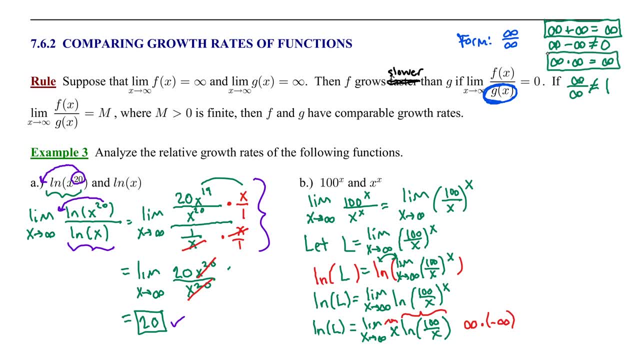 be confident of is when you have the product or sum of infinity. You can go ahead and make your conclusion there without any further analysis. So let's see where we are. We have the natural log of L equals the limit as x approaches. Oh, let's go ahead and. 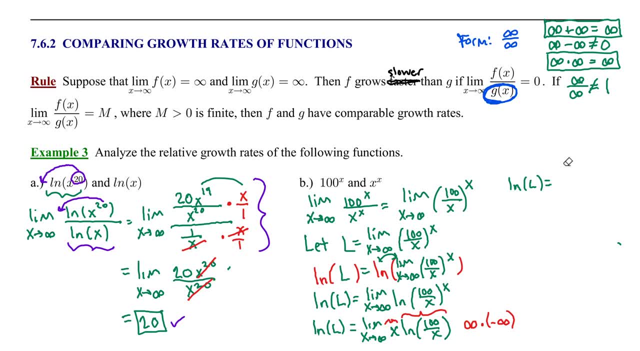 evaluate the limit We figured out. this limit is infinity and in particular- let's be careful here- negative infinity. Now, how in the world am I going to evaluate this? Well, we're going to use some unofficial notation here. e to the negative infinity.